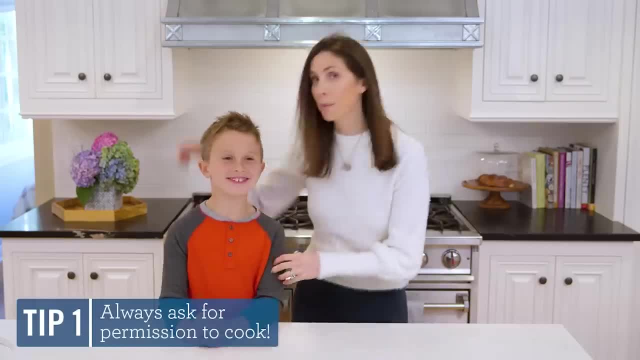 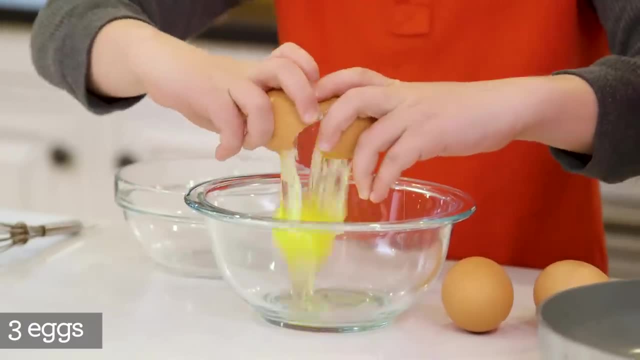 and these really yummy sticky buns. Alright, good luck. I'm going to be right over there, Alright, so first we're going to make our scrambled eggs. I'm really hungry, so I'm going to do three. So now I'm going to go ahead and wash my hands. 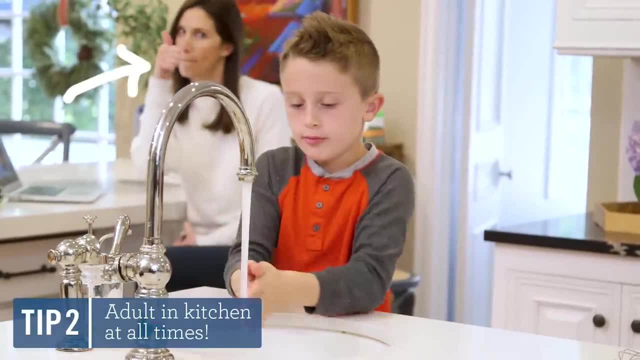 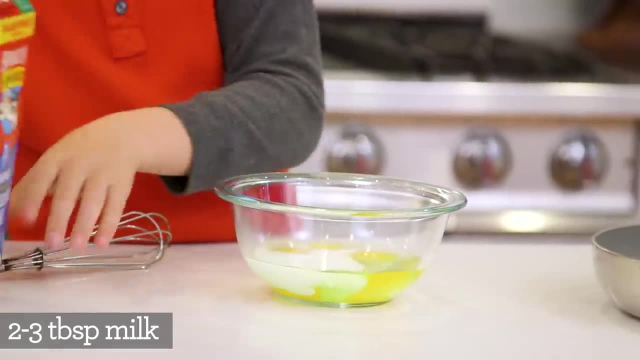 You want to wash your hands because the eggs have lots of germs in them. Okay, so now we're going to pour some milk in. This kind of makes it a little like the eggs, a little fluffier. So now we can start whisking this. 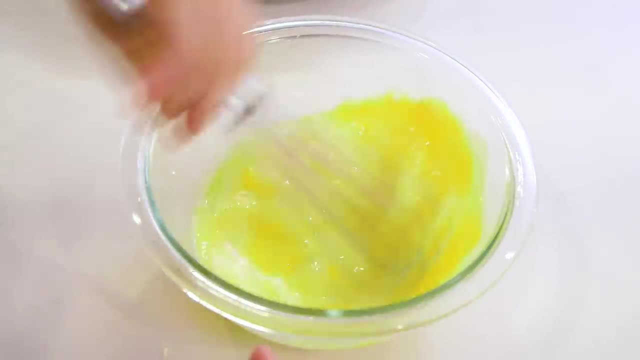 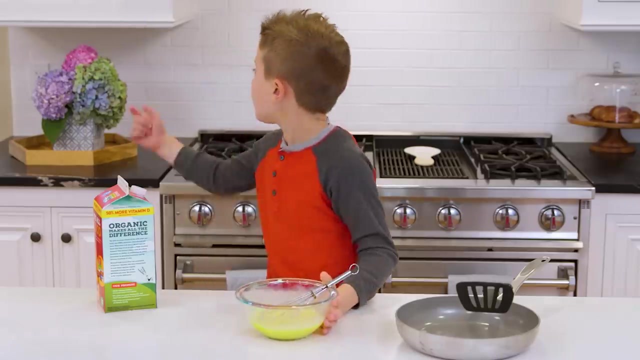 You need to be extra careful if you're using a small bowl, because it's really easy when you're whisking for it to get out of the bowl. I need the camera to follow me because I'm going to bring it to the sink to put this on. 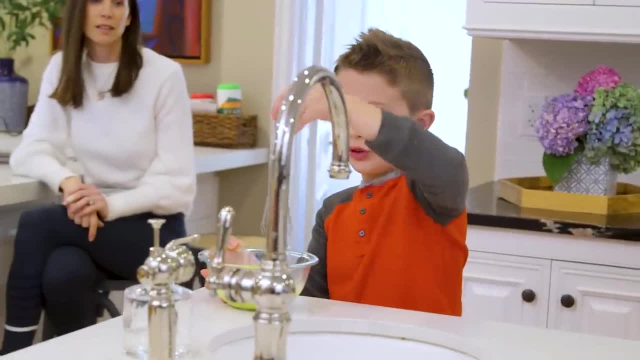 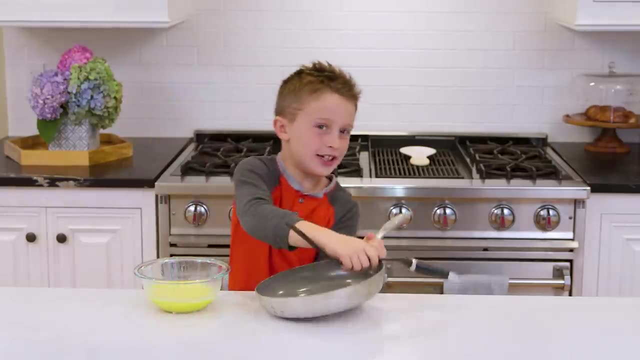 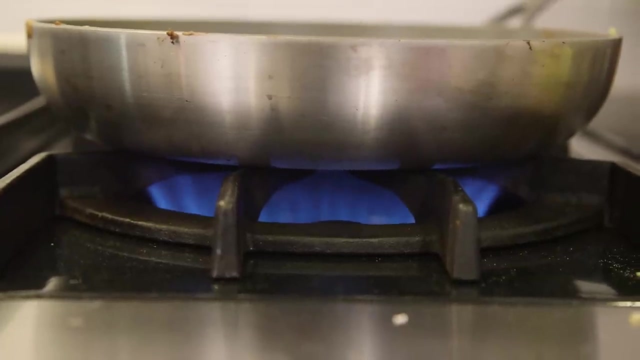 I'm going to bring the bowl and the whisk over so I can wash the whisk. So now we're ready to put the eggs on the stove and get cooking. We are going to turn the stove on, bring it to light. I'd say that's about good. 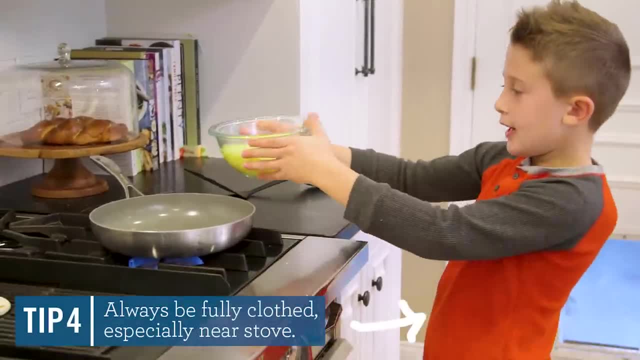 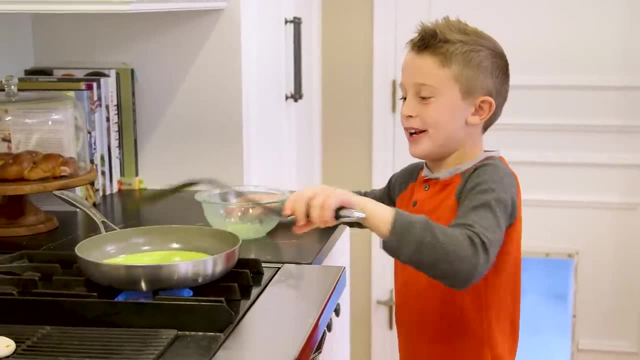 We're going to go ahead and pour the eggs in, And now we're going to wait a little bit. This is my least favorite part: waiting for the eggs to be ready. It takes a little time, but once you see it's kind of coming up on the sides. 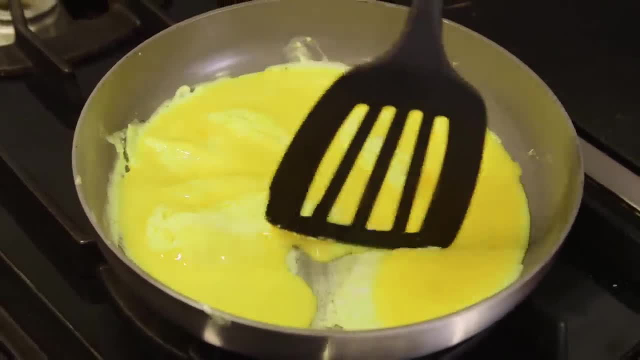 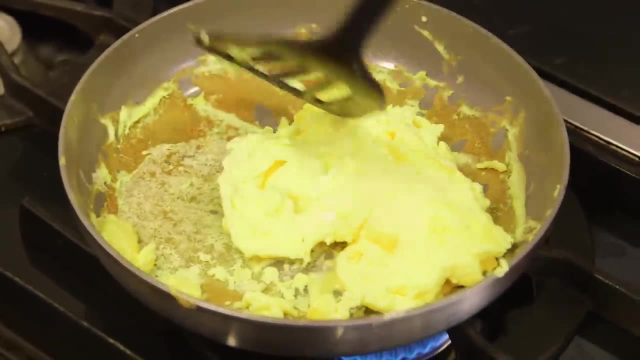 it looks a lot like eggs. Now I think it's time for us to flip it. You want to get all the way under to the other side, and you're going to flip it. So I can turn this off. Mom, I turned the stove off. 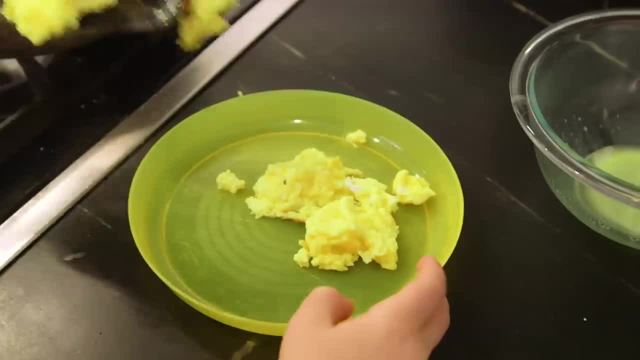 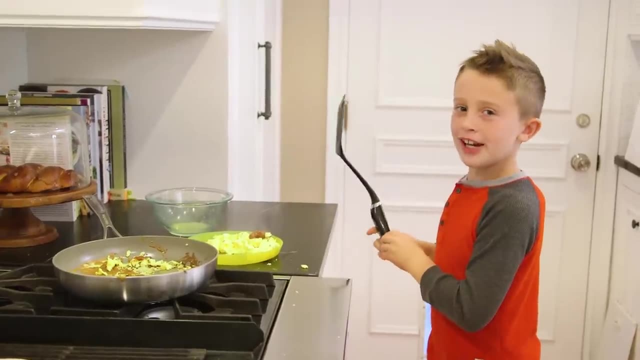 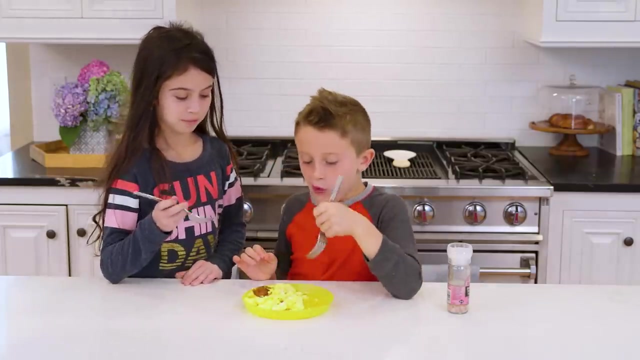 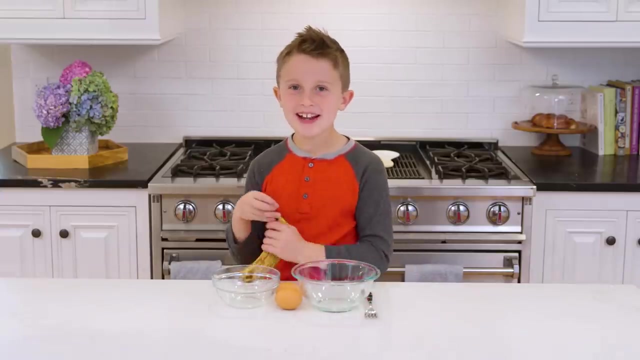 Here's the best part. Now we get to put them on the plate. Oops And voila- scrambled eggs. Avery, come, have some scrambled eggs with me. Mmm, This is the best part, definitely. Now we're making the two-ingredient banana pancakes. 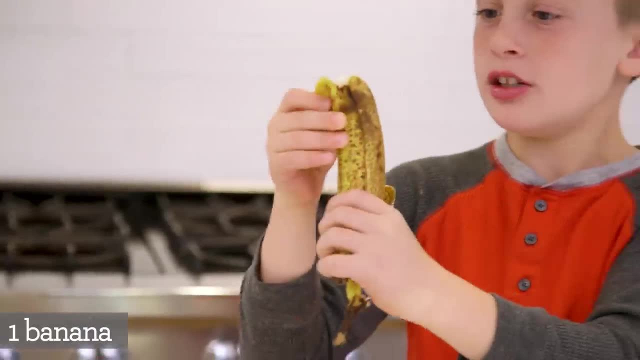 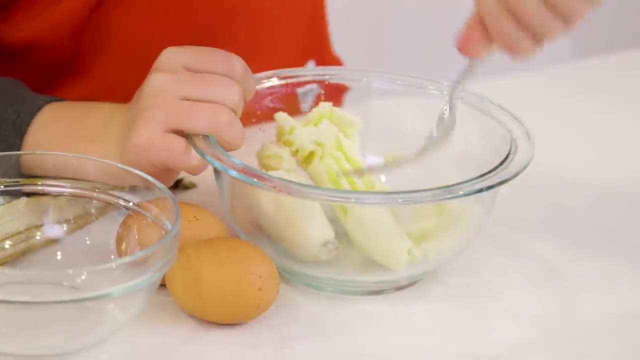 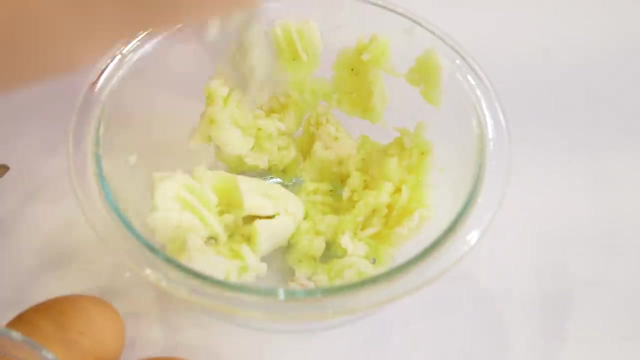 So now we're going to open this banana- Oddly satisfying- So now we're going to put it in the bowl and smush it. We have to smush this really really well. These are when muscles come in handy. I'm good at this. 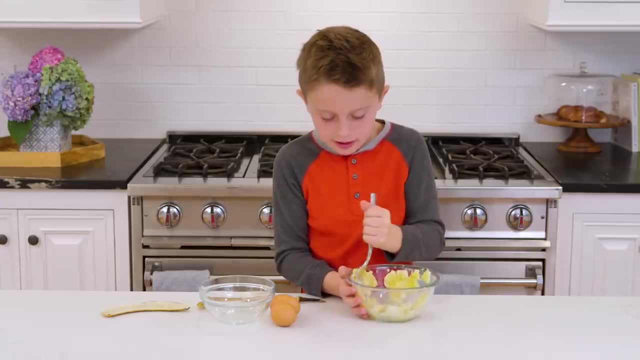 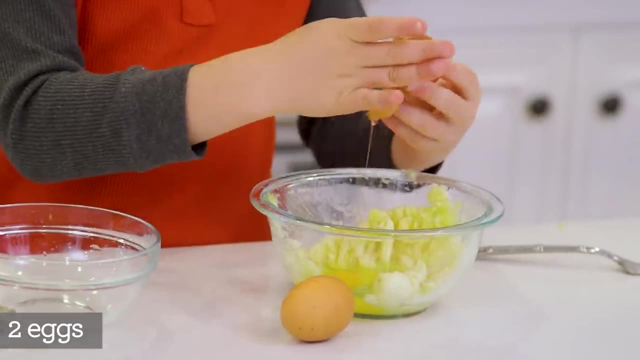 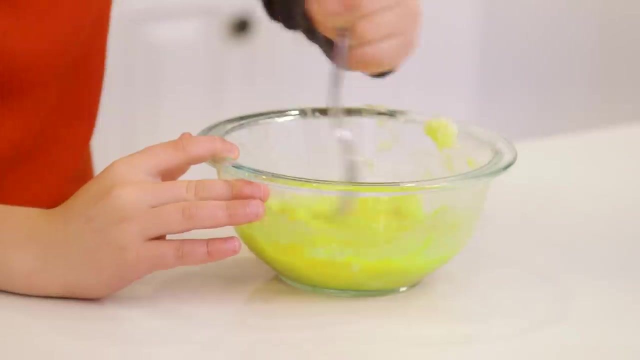 I'm better than my mom at cooking. I think, Okay, So now the same thing as the scrambled eggs: Crack this egg, Now the next egg. So now we're going to whisk And you can also go around and if you see anything that you didn't smush. 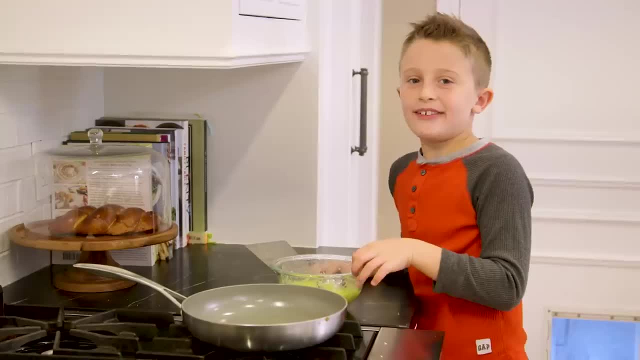 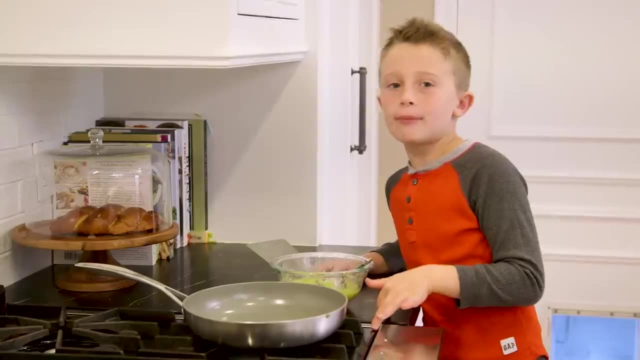 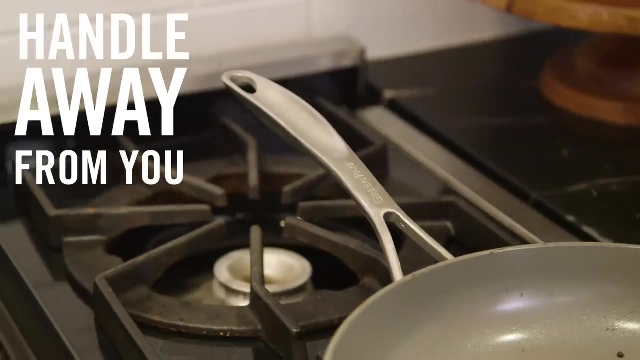 you can go and smush it again. So now we're going to cook the banana pancakes. So I have a couple tips for you that my mom and me discovered that they really help. The first one is just a safety tip. This should never be facing you. 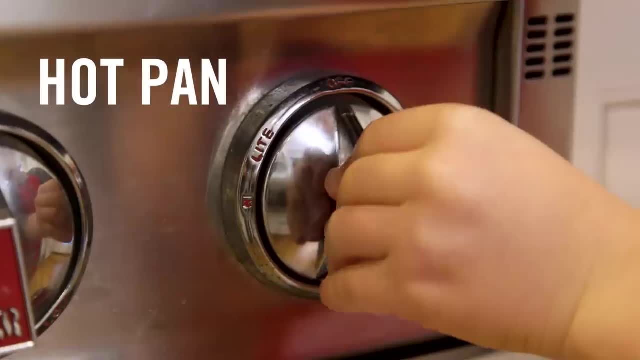 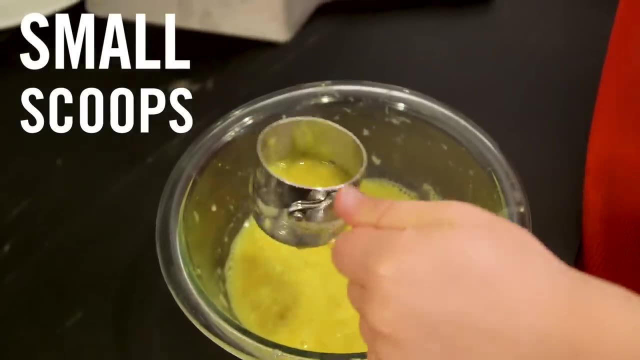 And also you want the pan to be really warm. And next you need really small scoops so that it'll be easier to flip, and a really thin spatula so it'll be easier to flip. So let's pour this baby in. 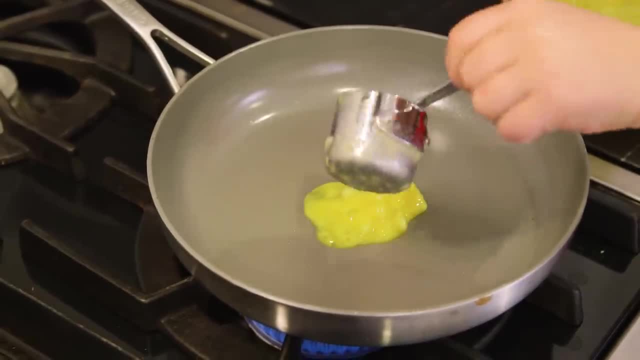 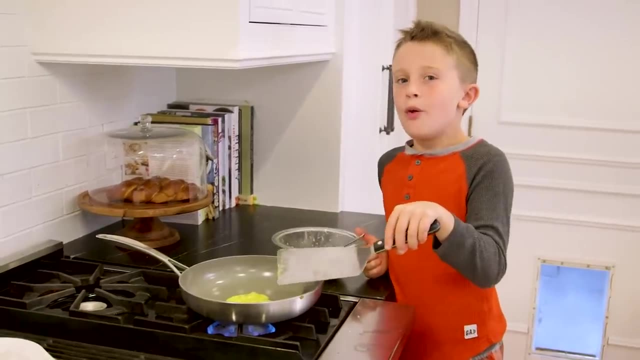 We're going to do it right in the middle, So now we're waiting for, like, the edges to get cooked. This is something me and my mom had to practice a bit. We learned you can't flip too early. Ooh, that looks pretty good. 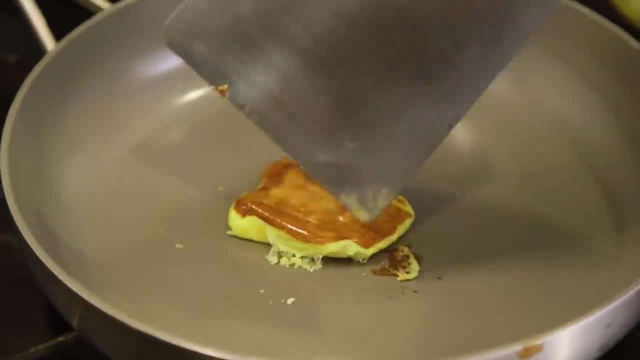 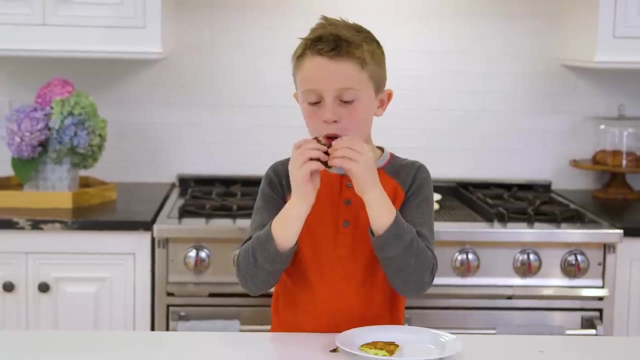 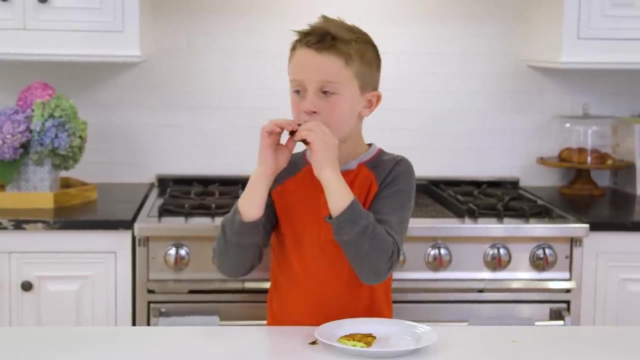 Now you need to really get completely under it. I think I did a really good job on that one And that's a wrap. on the banana pancakes: Mmm, They could use a little maple syrup, but they're good plain because they have lots of flavor in them. 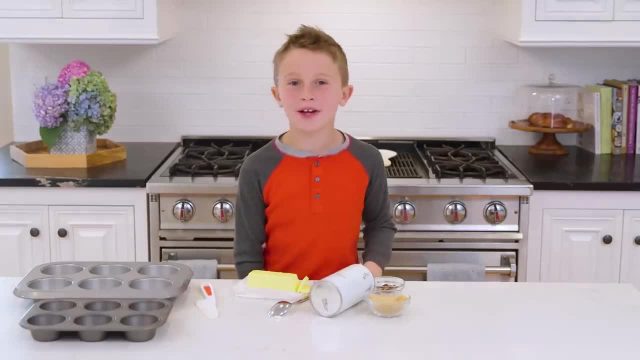 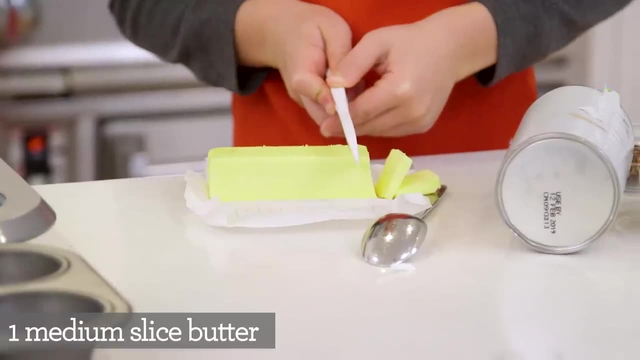 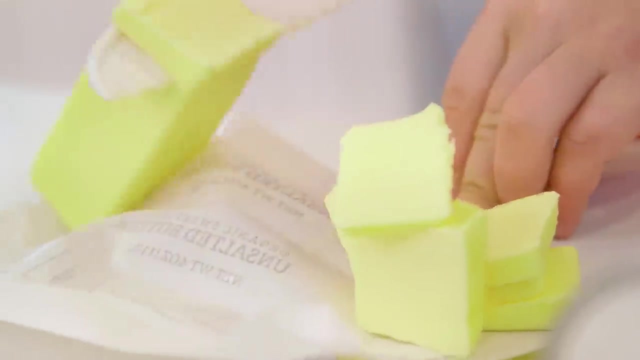 Mmm. So now for our last kid recipe. we're making semi-homemade, super yummy sticky buns. So the first step is cutting the butter, but you need to cut the butter really big And I'm using my kid knife. 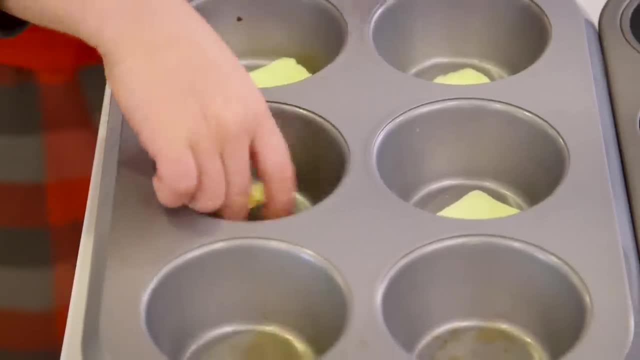 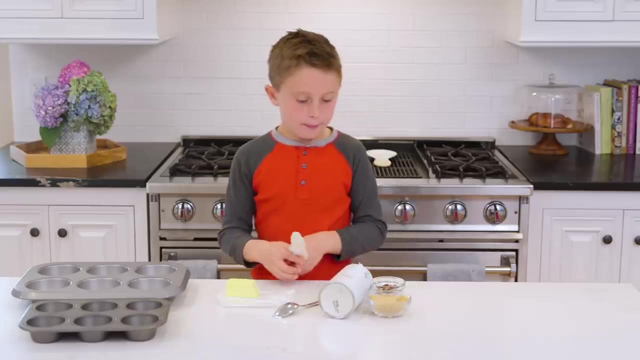 We're going to fill it up, so we're going to put one in. I like this part because you get to get your hands all messy and I like getting messy. We're going to put some brown sugar in. I put lots of brown sugar in.